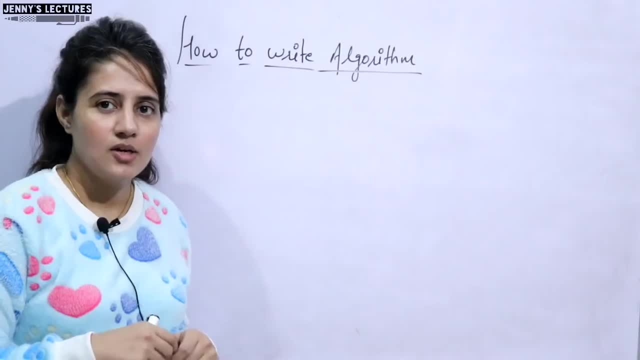 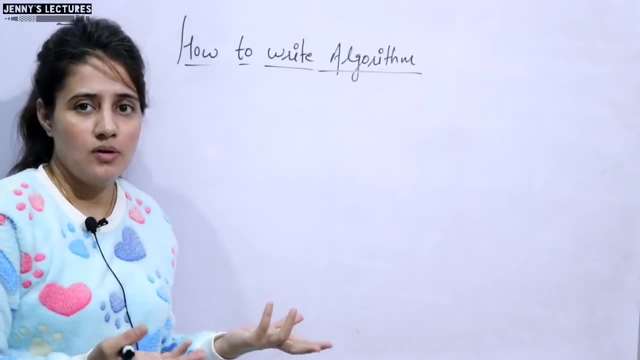 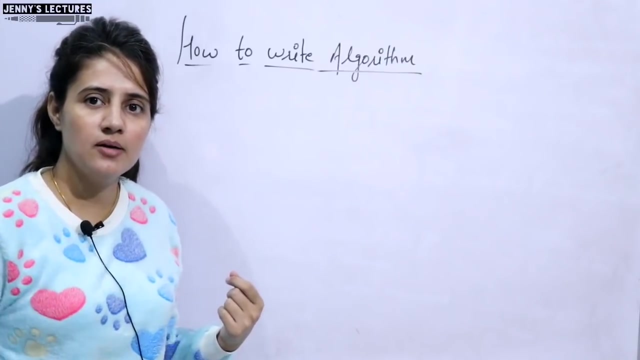 you in the description box of this video. you can go and check out there. So now let us take one example. I am going to take simple example: sum of two numbers. right, the procedure is what like? you need to take two numbers, input of two numbers, then add two numbers, a plus b, then print the sum. 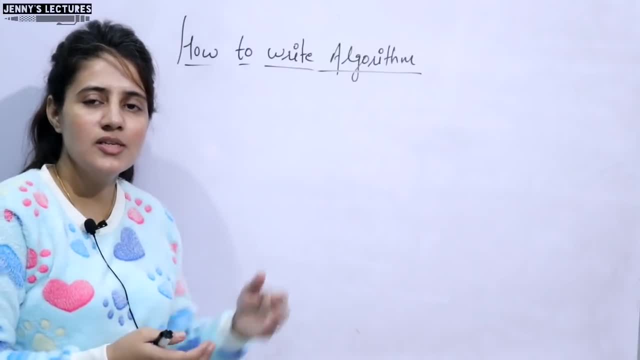 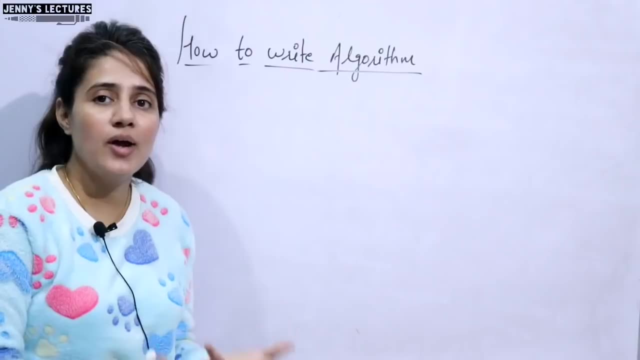 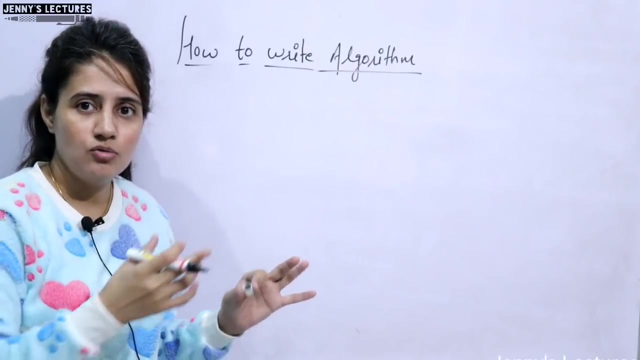 right, these are the steps. So algorithm is what? Obviously, these are sequence of instruction or sequence of steps to solve a particular type of problem. right now, how to write an algorithm. see, generally we write what. there is no standard rule for writing algorithm. like you have to follow these rules, only you. 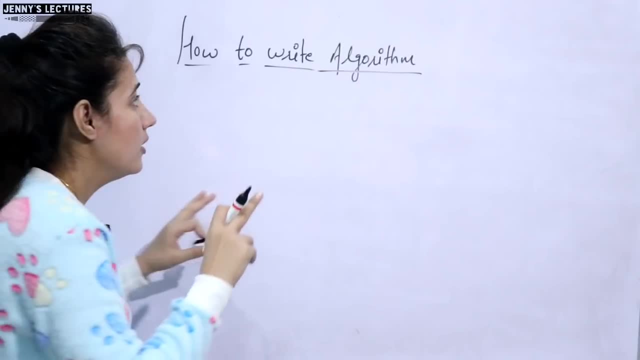 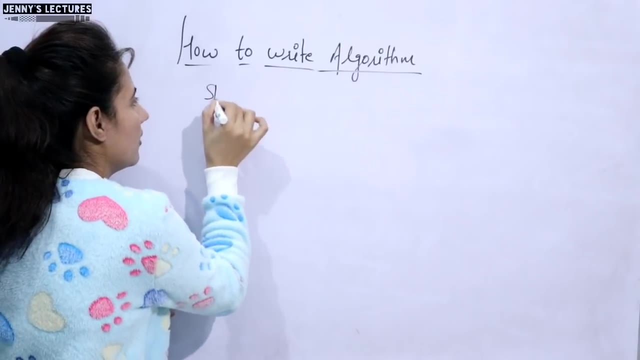 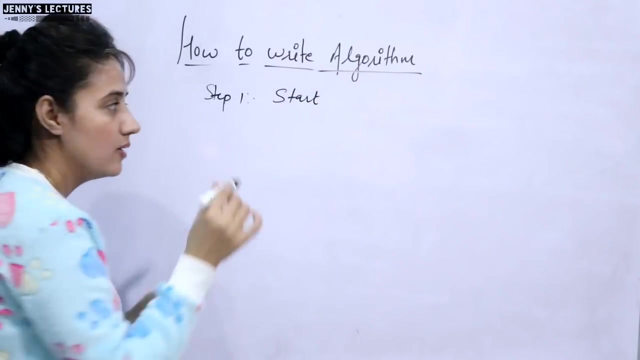 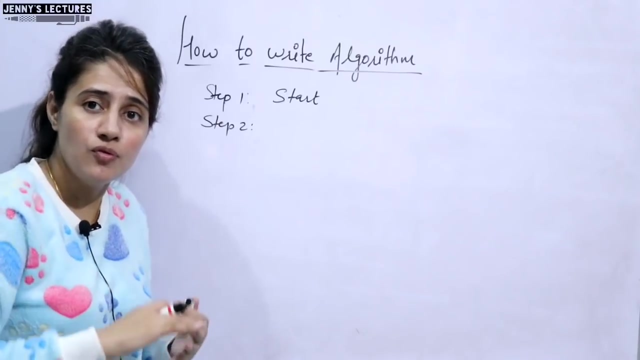 have to write this type only that. thing else also will discuss. so first thing is: generally we write numbering of each instruction or each step, like: first is step one and in step one we write what start, right, then step two. now for adding two numbers, you need two numbers, right? so you need input of two numbers. so here: 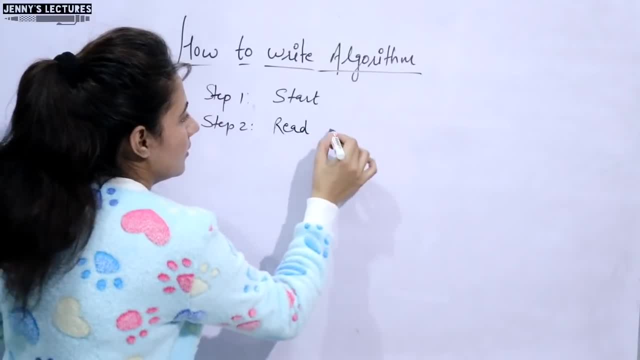 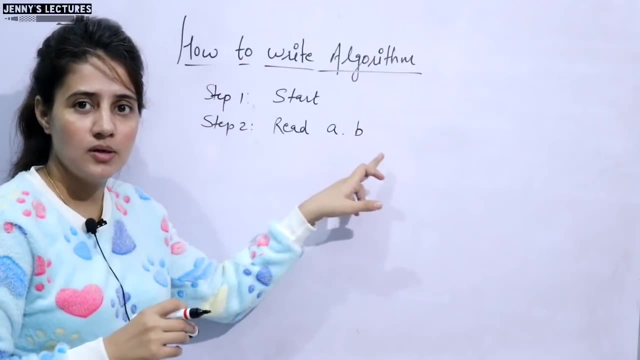 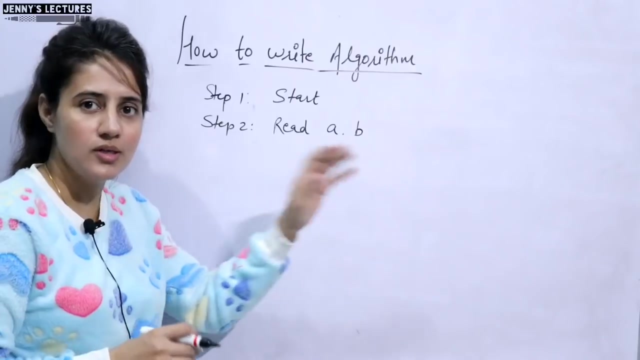 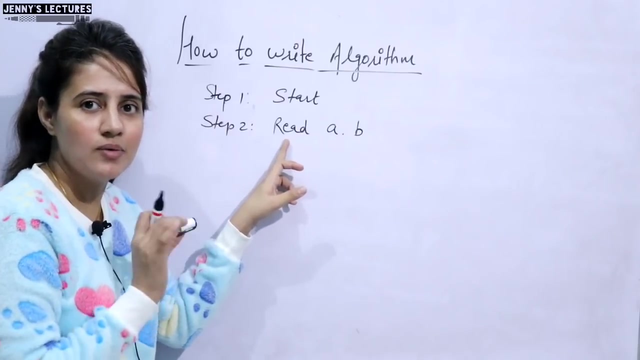 you can write read A and B, or you can write input two numbers, A and B, or you can write enter: enter A, B. yeah, enter num1, num2. it's up to you, right? but see, here I am writing either read or input or enter. but whatever I am writing, you are able to understand, right. 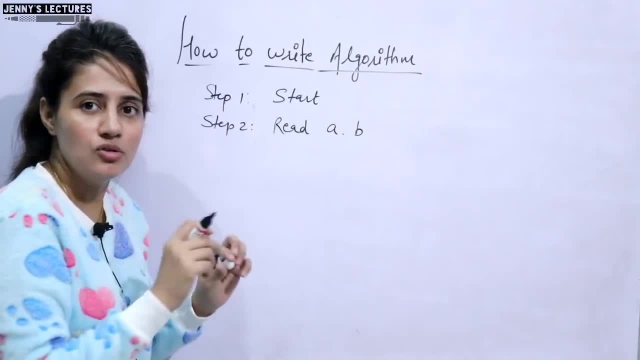 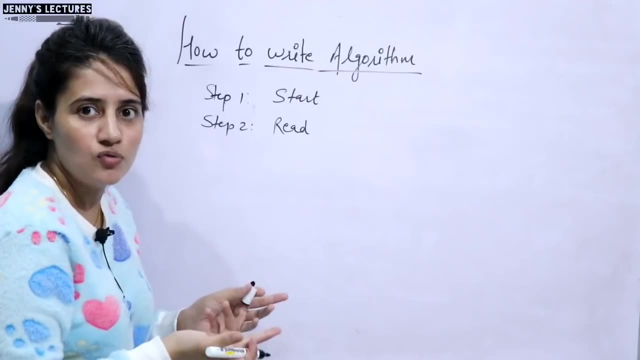 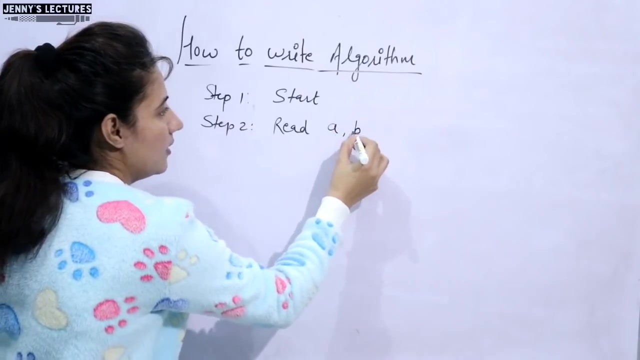 that is the main thing. each instruction should be clear and unambiguous. it's not like that. I am simply writing read. now, this is what we are not able to understand. it is ambiguous statement. but if I am writing read A and B, it means what I am reading: two numbers. I am inputting two numbers, fine. 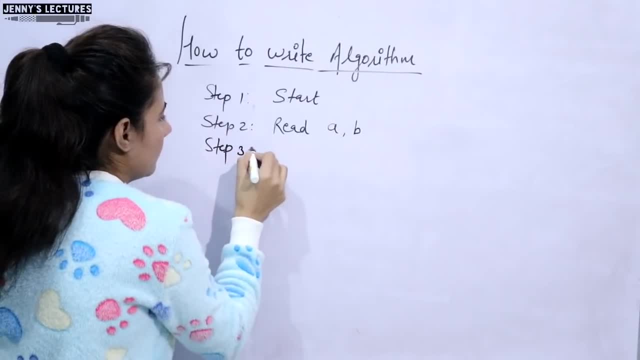 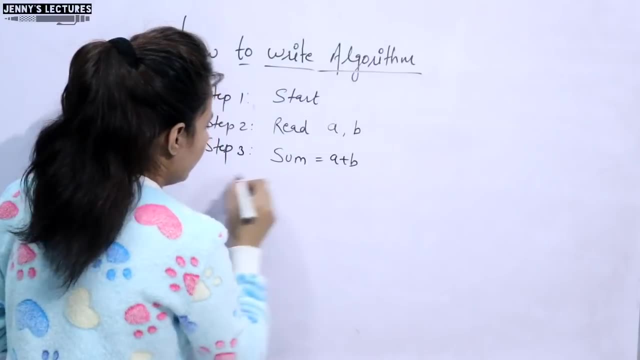 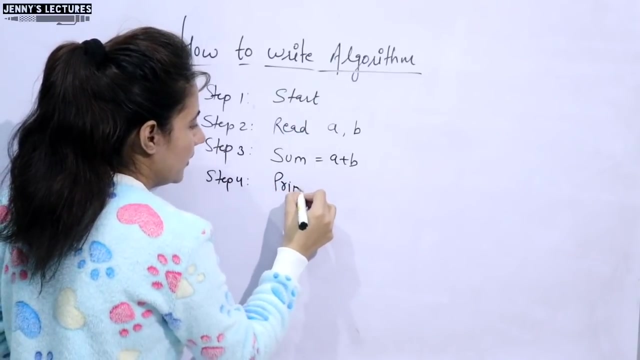 now next step. now we need to process on these inputs. process is what you need: to calculate sum. now in step four, what you will do, just you will print sum. you can all write here: print sum. and step five is what stop or here you can also write. 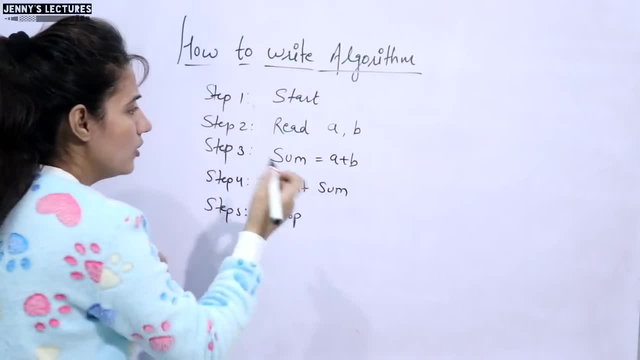 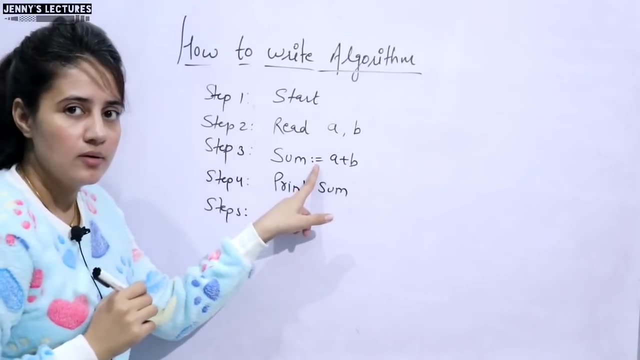 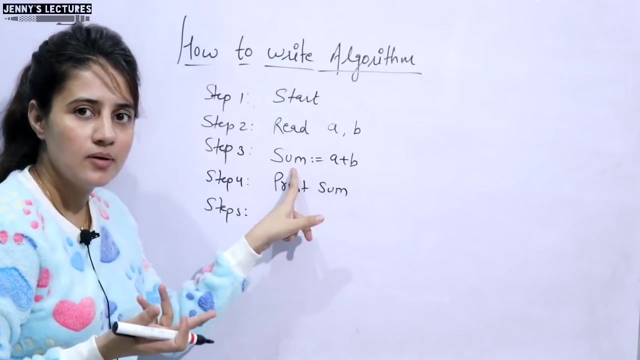 end. so this is simple example. now, here you can also write something like this: the symbol is equal to. so here you can also write like this: in algorithm you can also write like this: this is the same. I mean the meaning is same: sum of A plus B, and that value would be assigned to sum. now, if you will say you haven't, I 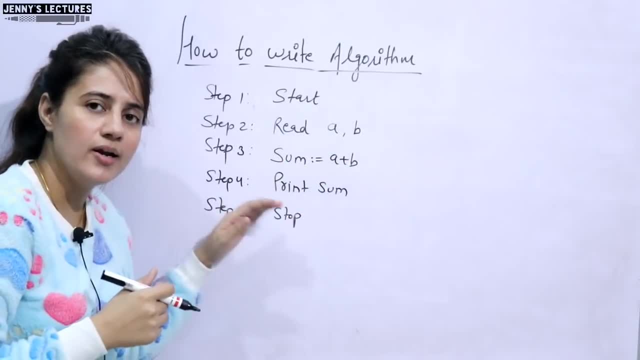 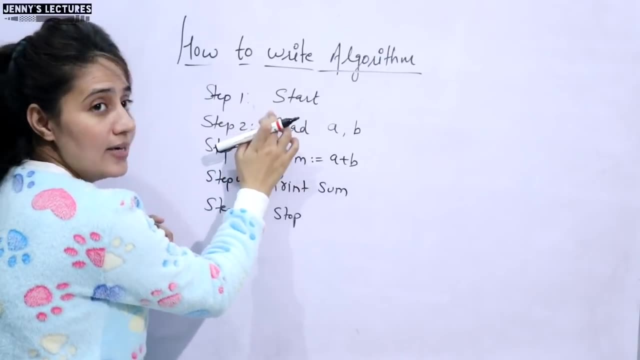 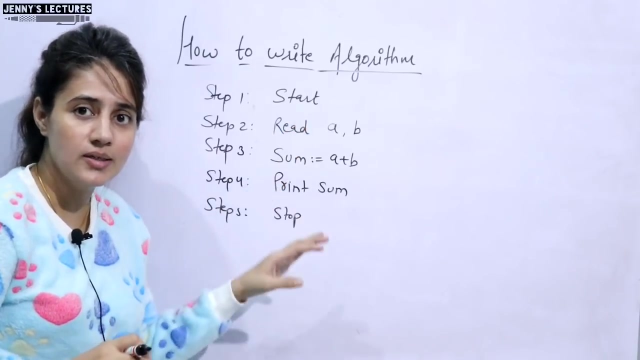 haven't declared A, B or sum. so when you write algorithm then no need to declare any variables. but if you want to declare, you can also write here after start and declare variable A, B and sum. that is also fine. that is why I have already told you that there is no standard standard rule for writing algorithm. 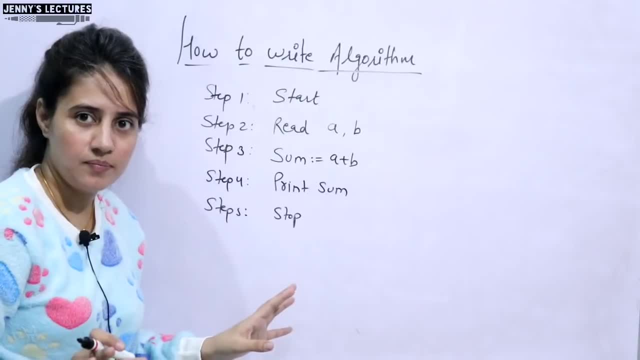 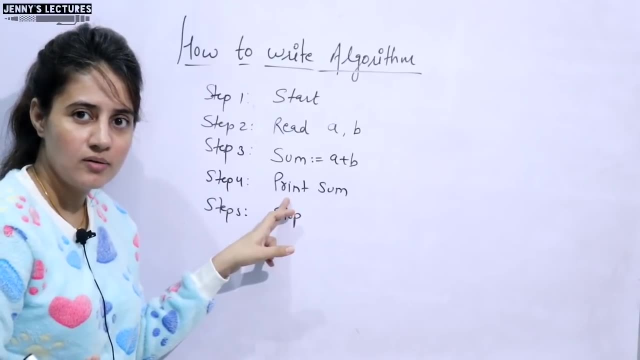 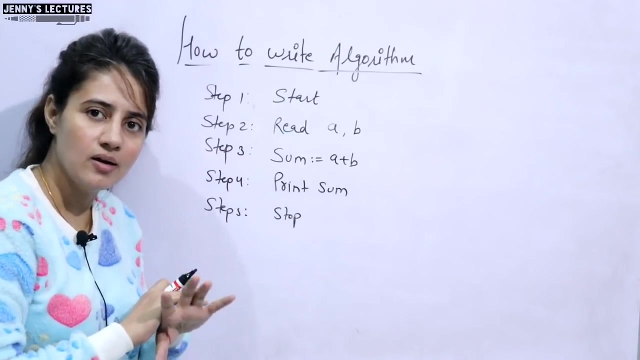 right. if you are not declaring these variables, that is also fine. here you are writing print sum. here you can write output sum, that is also fine. but whatever you are, you are going to return- that should be understandable- that each instruction should be very clear and unambiguous. that is the main thing. 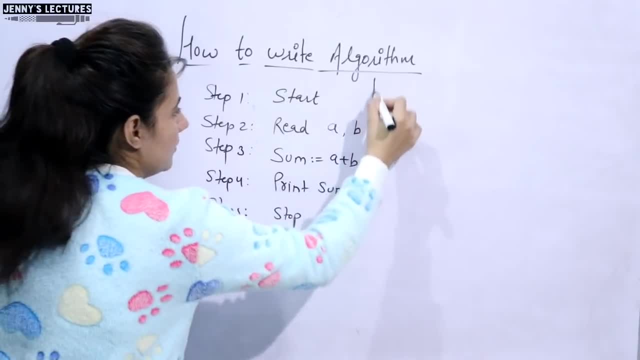 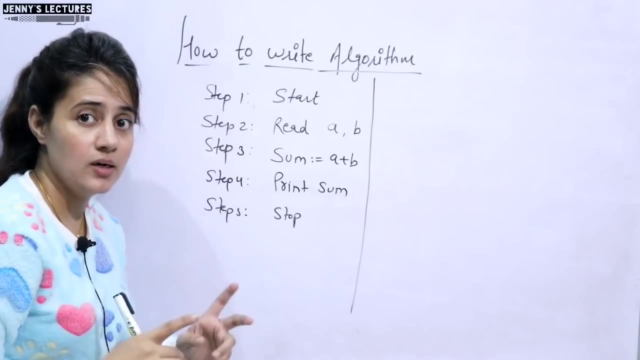 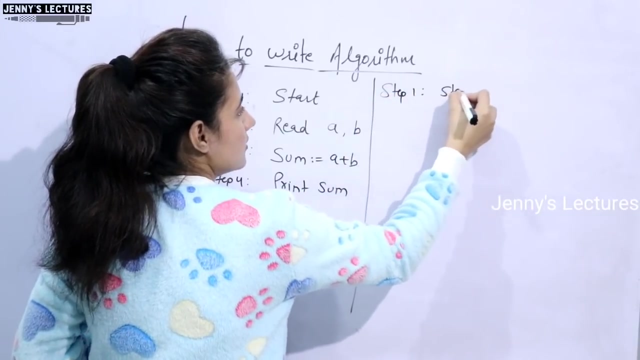 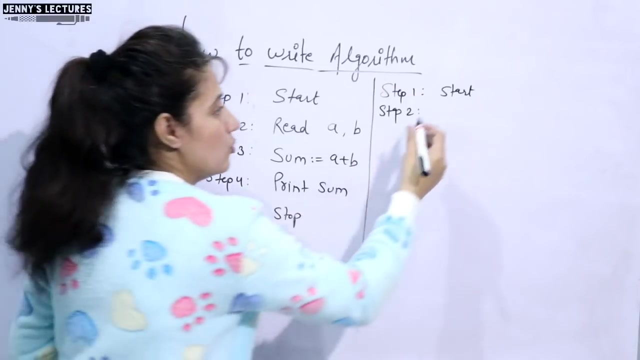 this is a simple example. now let me take one more example like: suppose, if you want to write an algorithm for finding out a largest among three numbers, then here obviously you will need if-else statements. so first is same, you will write step one and start step two. three numbers you need, right so you can write. 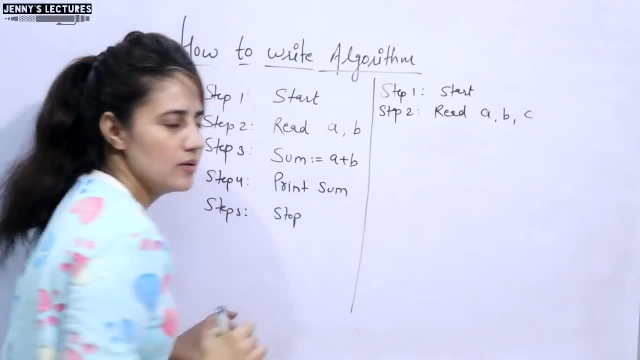 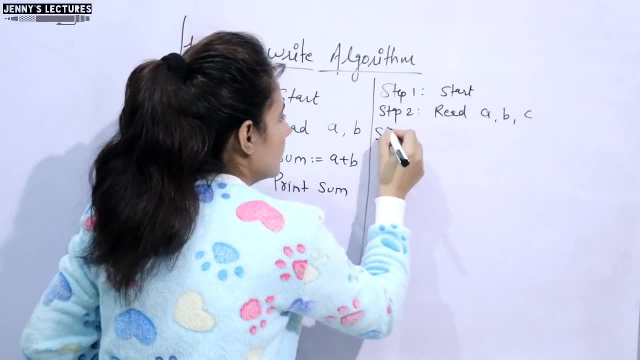 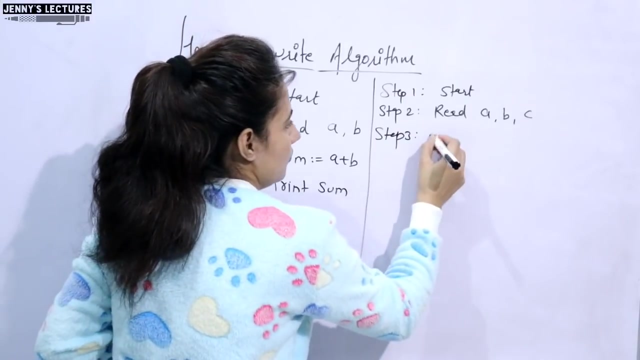 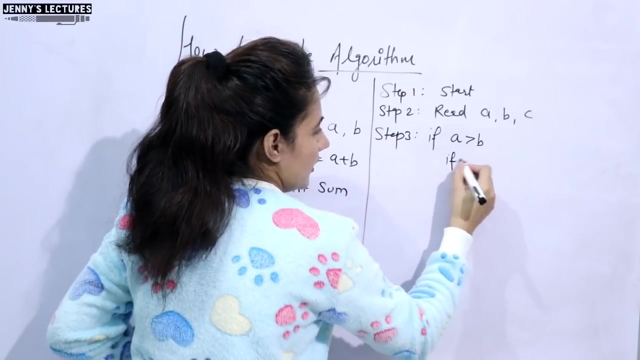 here: read A B C. fine, or you can write enter A B C, or you can write input A B C. now step third is: now you need to check which one is largest. so how can you check? like, if we write if A greater than B, then here also you will check A greater than B again if 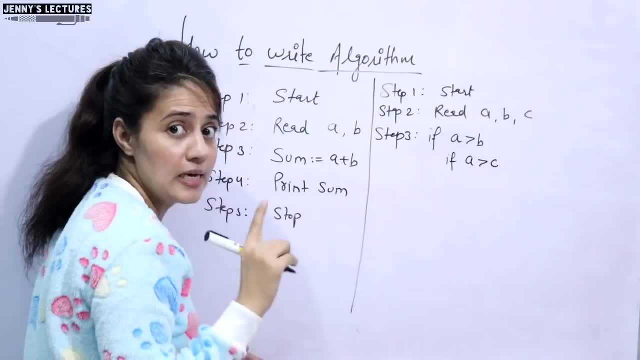 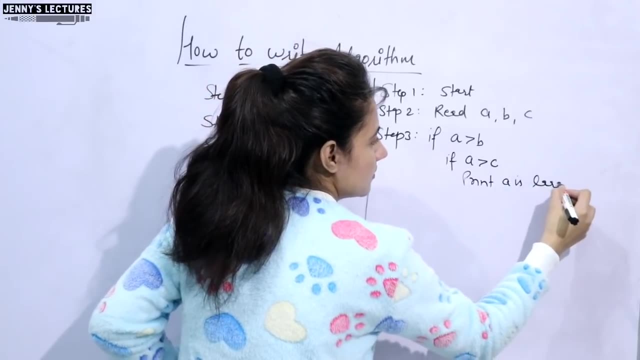 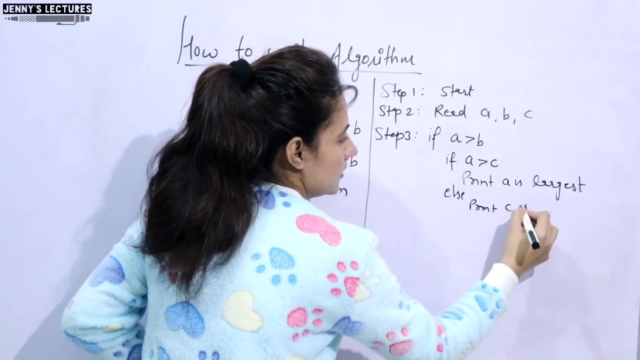 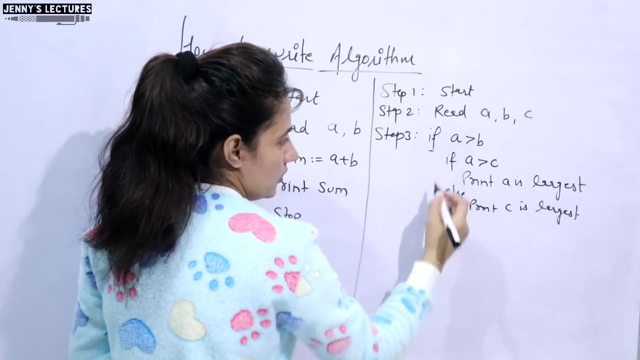 A greater than C means largest is what A. so here you can write: print A is largest, right else, print C is largest. I hope you are getting why I am writing C is largest right now. if-else for this, if-else will check if B greater. 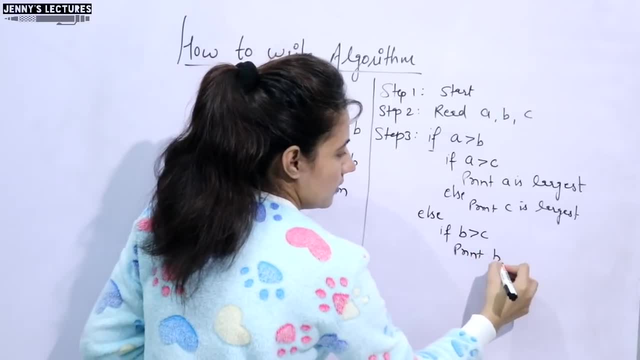 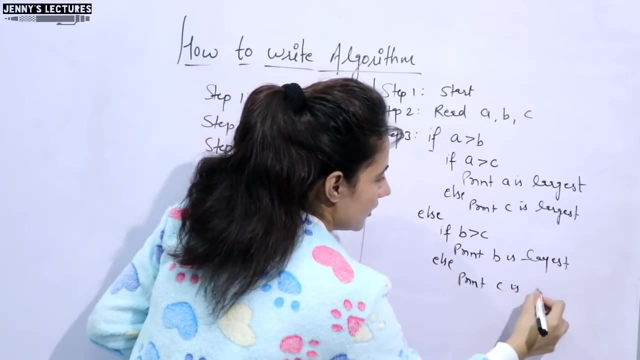 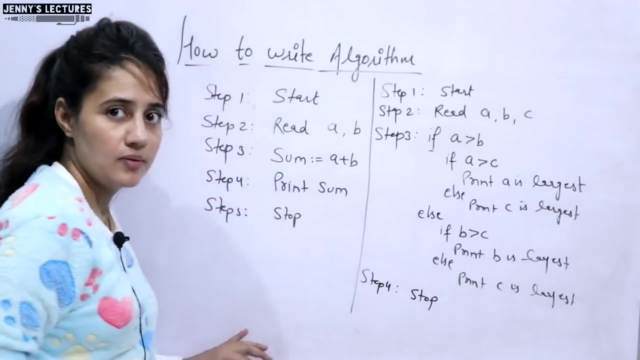 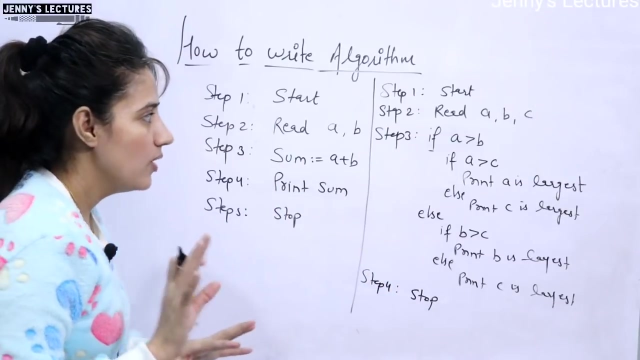 than C, then you will print B is largest, else print C is largest. and now it's done. in step 4 you can write stop or end. this is one way of writing algorithm for finding largest number. there are multiple ways. second way, maybe I am writing step one: same start in step two. 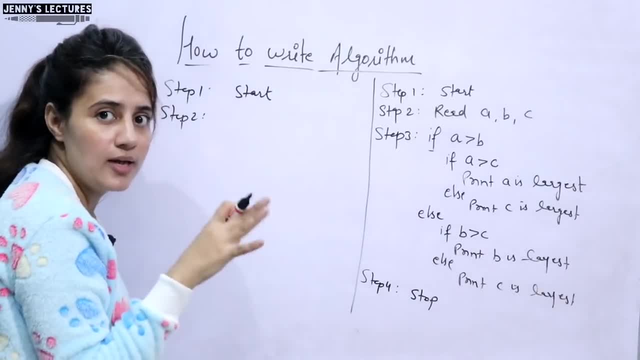 you have to read input. if there is any input in algorithm, see in properties. you have to read input if there is any input in algorithm, see in properties. we have seen there can be zero input or more than zero inputs, like 1, 2, 3, so here: 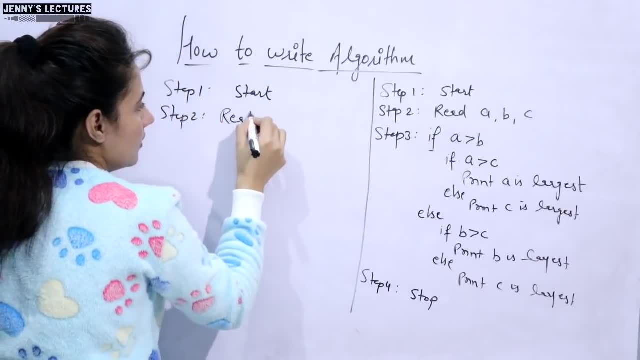 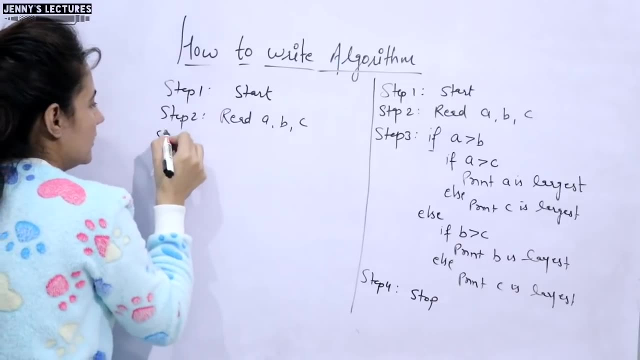 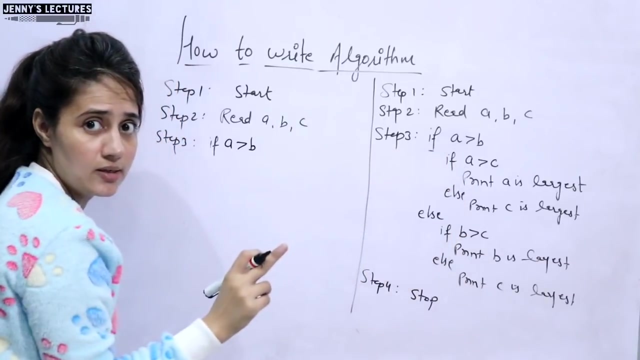 we have three inputs so you can write: read A, B, C or num 1, num 2, num 3, up to you. these are variables. name of variables. in step three I can write if A greater than B. see in one step only. I have written all these, but here you can write down in: 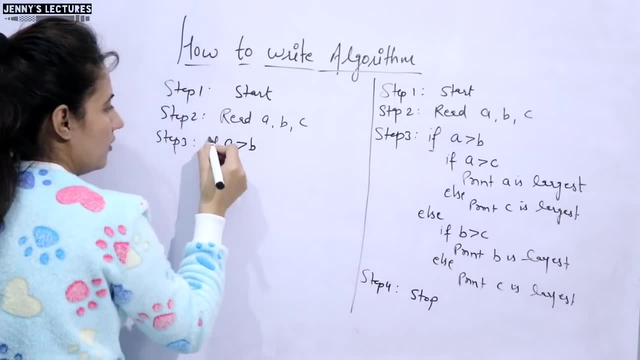 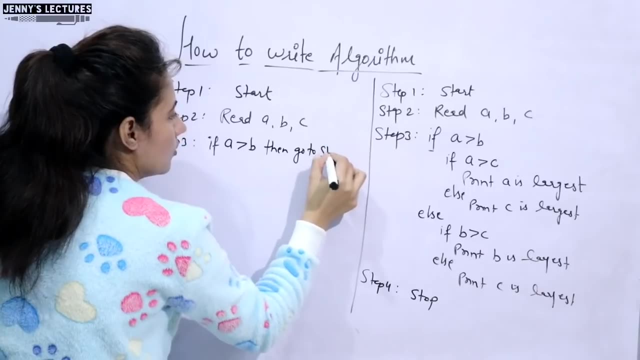 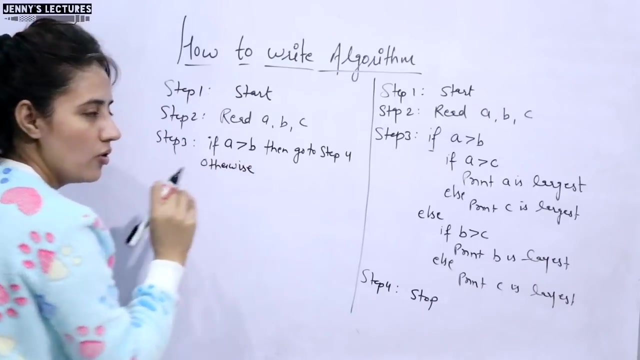 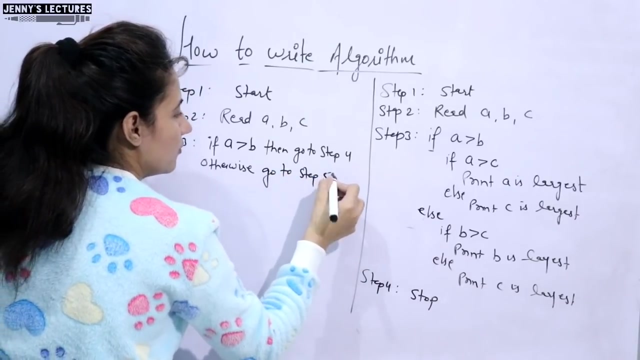 different, different steps. so what you can do. suppose I am writing: if A greater than B, then go to step for like next step, otherwise see when you are writing algorithm. then at place of else, you can also write otherwise, go to step 5. now step 4 is what? in step 4 I'm writing this condition. I'm checking this. 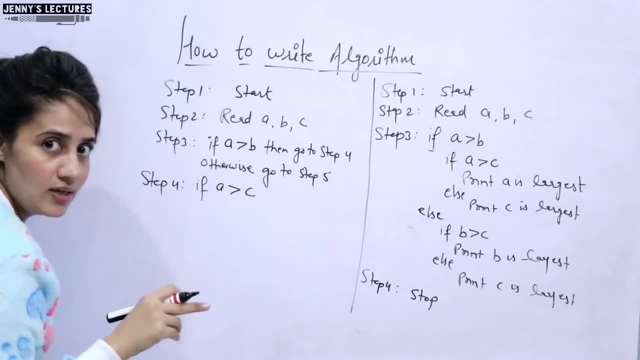 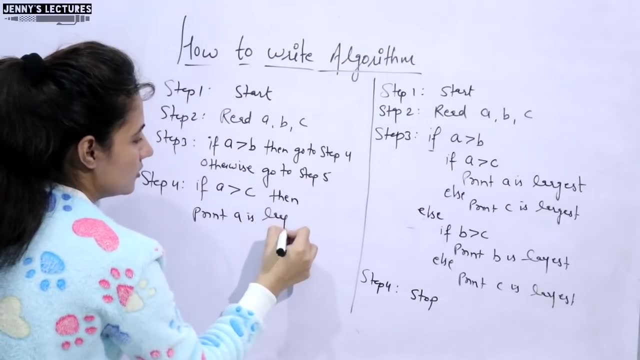 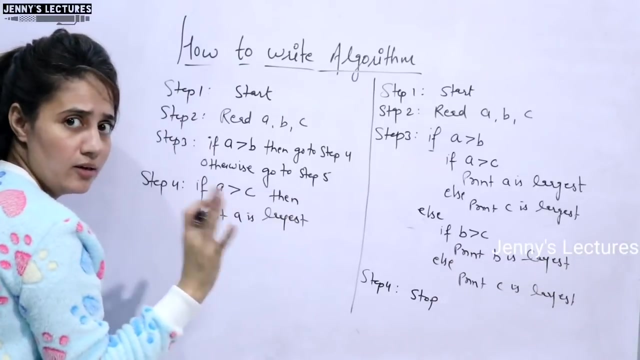 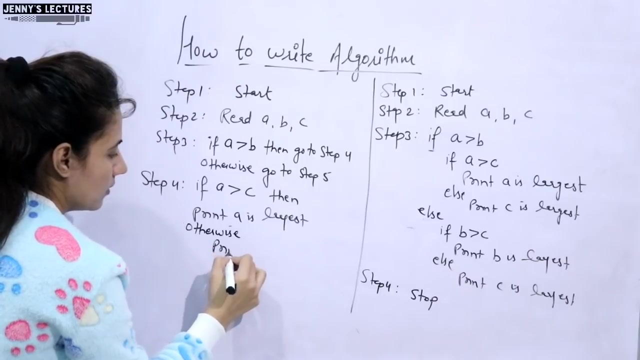 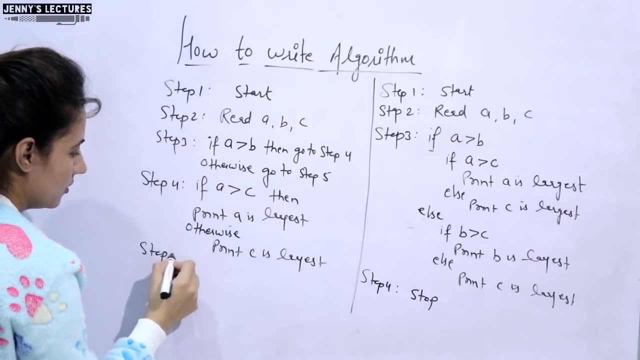 condition: if A is greater than C, then print A is largest. It is ok, You can write then. If you do not write, then it is also fine, Ok. Otherwise, print C is largest Right. And step 5 is what? This condition? I am writing in step 5.. 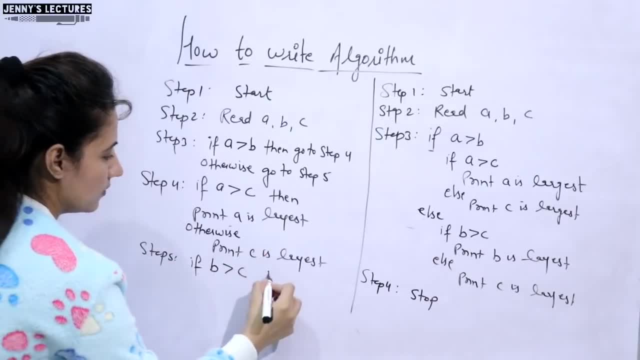 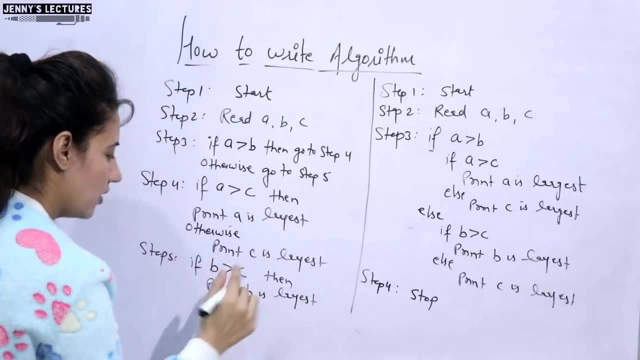 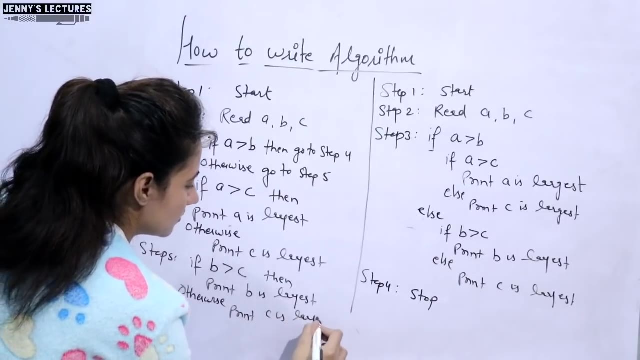 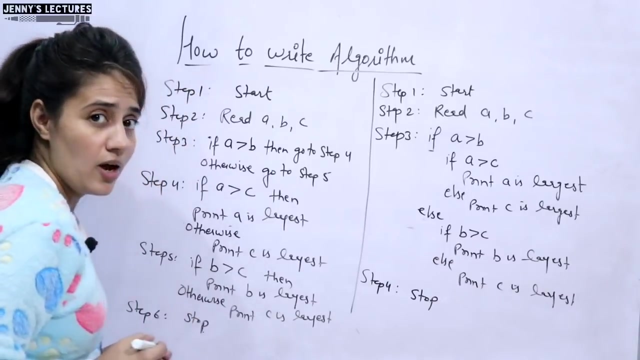 If B greater than C, then print B is largest, Otherwise, Ok, Print C is largest. And next step, step 6: here you can write stop or end. So this is how you can write algorithm, and algorithm is what It is, independent of any. 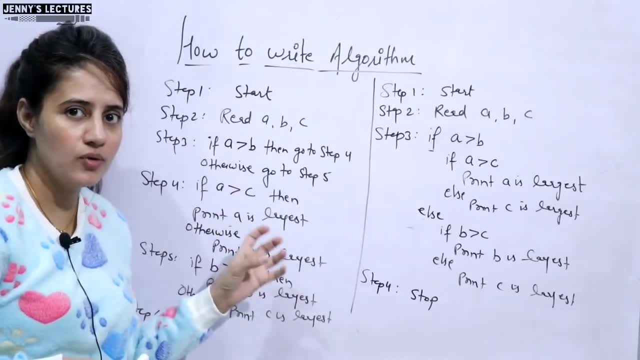 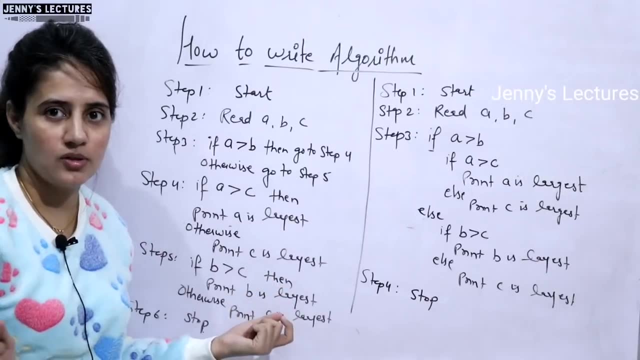 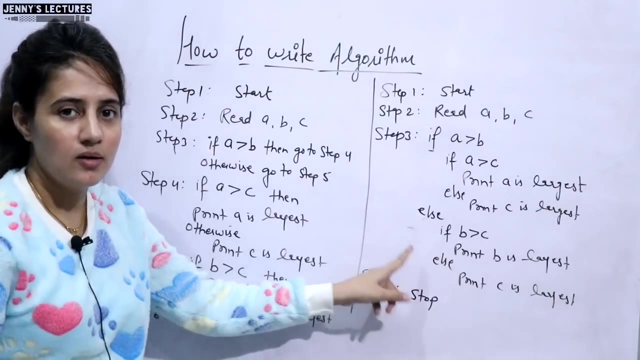 programming language. Simple, natural, in natural language. or you can say in English language: you will write down algorithm and you can implement the algorithm in any programming language. It does not matter that. if you will write this type of algorithm then you can implement in C, only right. And if you write this kind of algorithm you can implement. 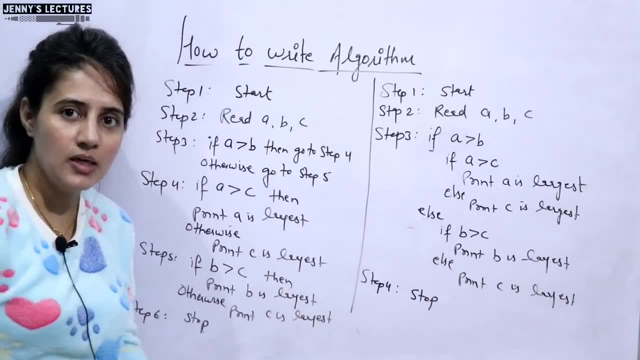 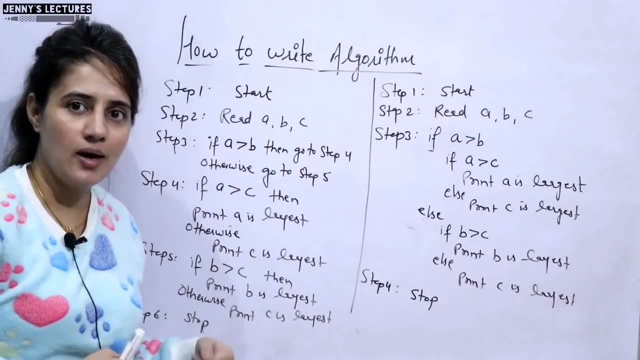 it in Java only Like the same example. if you want to prepare tea, then steps are what You will: add some water in a pan, put it on flame, then add tea leaves, sugar and milk and only then boil and your tea is ready. Now it doesnt matter that you are preparing. 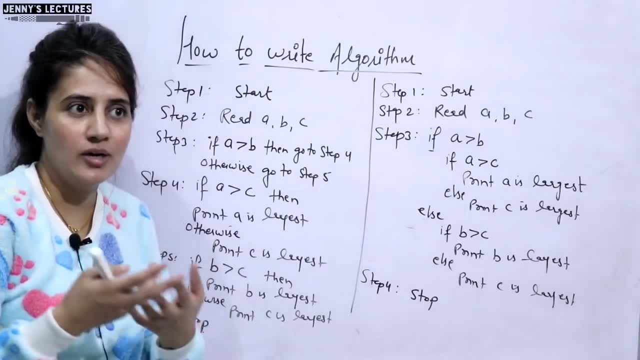 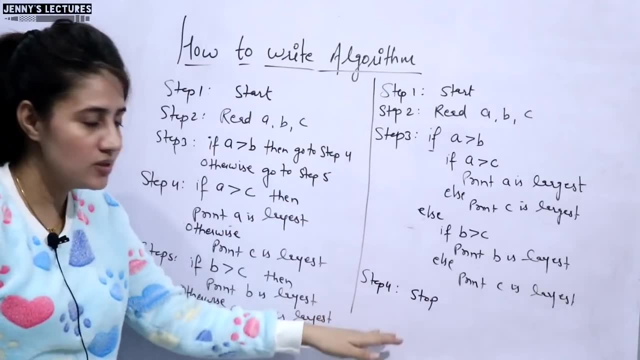 tea on gas stove, chula or induction or on heater right? Obviously, you have خ carte as same information. everything is up to the maker. Done steps would be same, So steps would be same. it does not matter. you are implementing this. 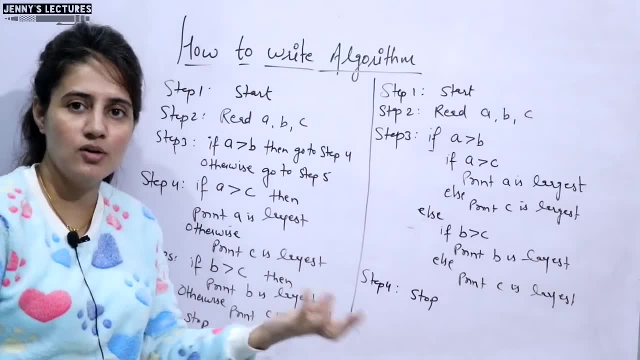 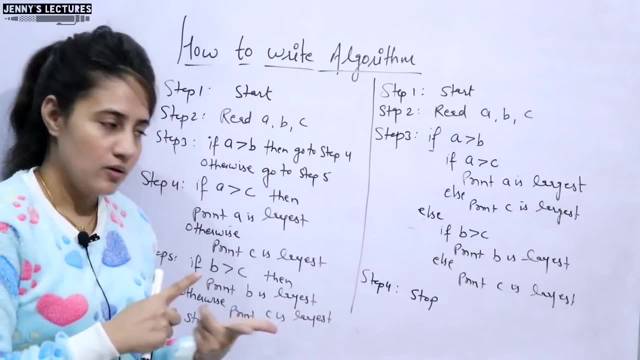 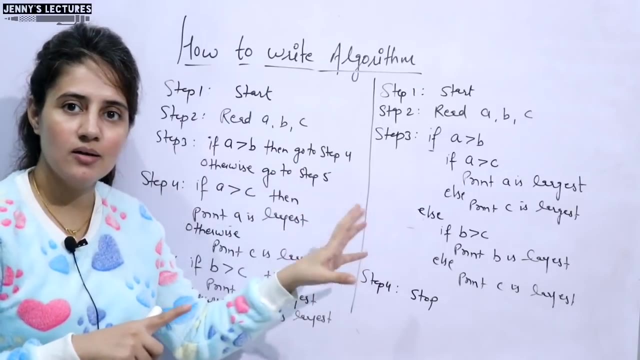 in C language, Java language, Python or dotnet or in any other language. But when you are writing algorithm you have to follow the properties. Input: there should be one output. input can be zero or more input. output should be one and every statement would be clear: have one. 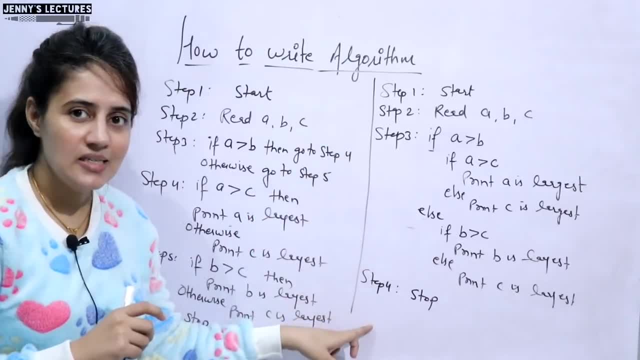 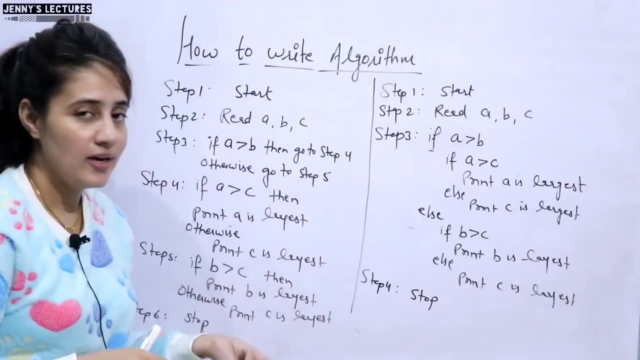 meaning unambiguous there should be. finiteness means finite steps would be there in algorithm. all these properties we have already discussed, So I hope you got how to write an algorithm. If you want to write any loop, like in loop, what you need to do within that loop, whatever. 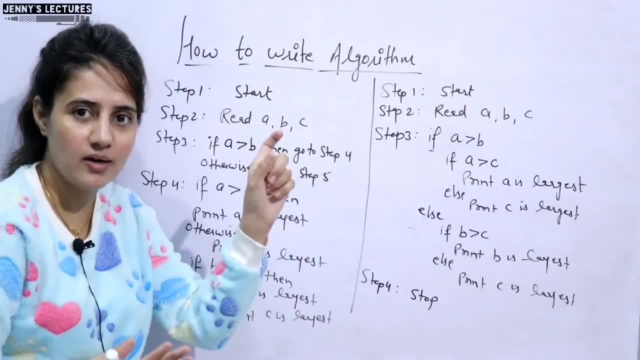 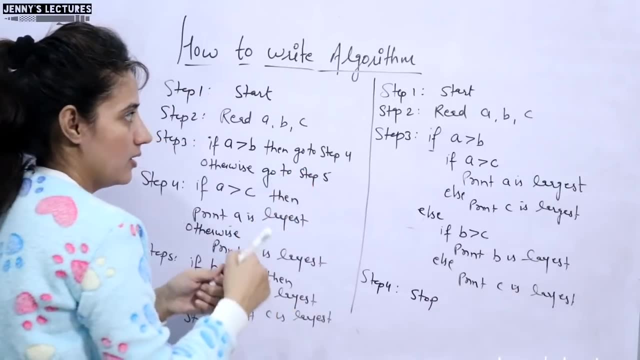 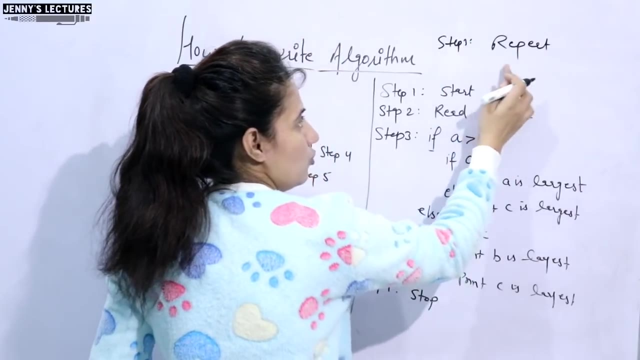 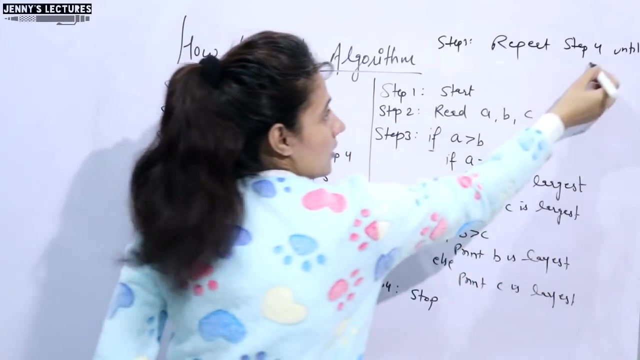 you will write those statements would be repeated, right? So you can write what simple repeat step, next step, like suppose here in this step I am writing: This is step suppose third, and I want to repeat next step, So you can write: repeat step 4 until the condition here you can write. condition means no need to write down brackets. 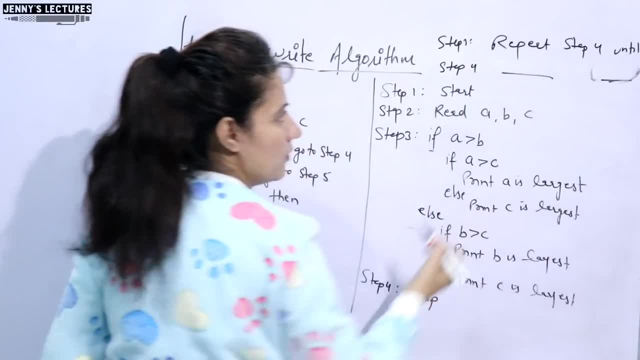 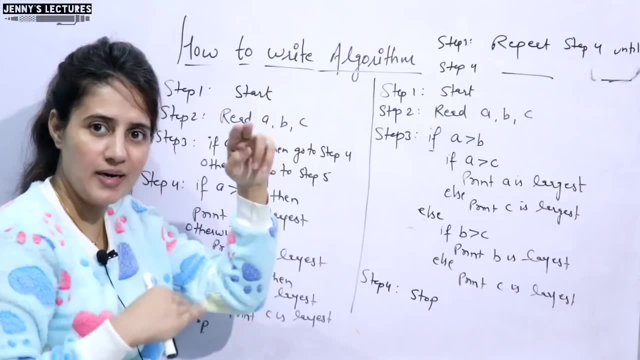 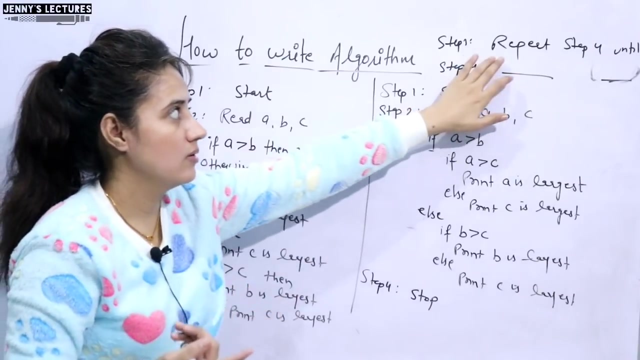 just write down condition. and next step is 4: you can whatever you want to repeat. you can write down here, Obviously, whatever you will, written in the loops, those in the those brackets, those statements would be repeated. till that condition you will give: that is true, right, So same repeated. you can also write this simple word: repeat, So that is.